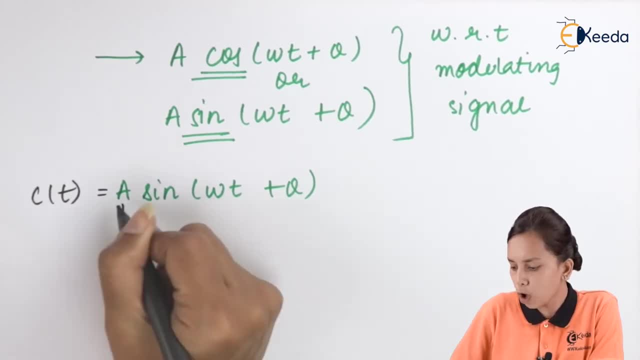 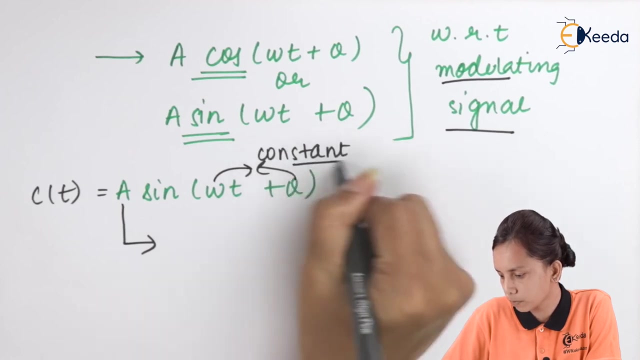 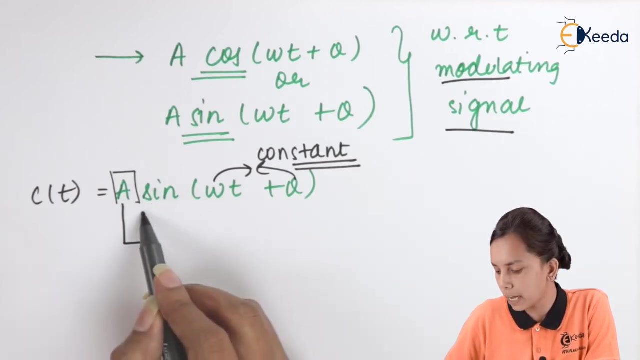 when we are saying that the amplitude of this carrier wave is changing with respect to modulating signal. such a signal is known as amplitude modulated signal. now we are keeping this omega and theta as constant, only This characteristic will change. Let us try to look with the help of a graph. 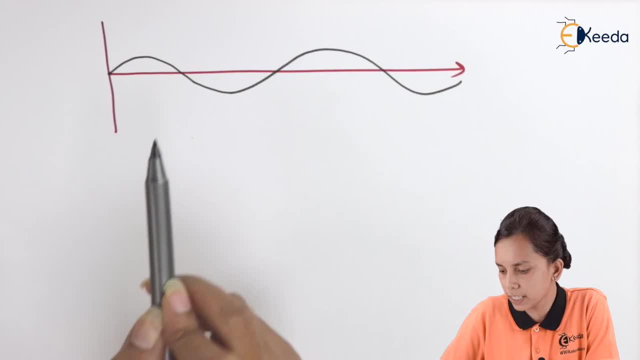 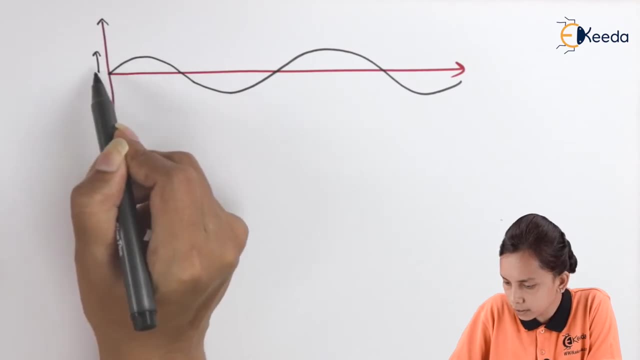 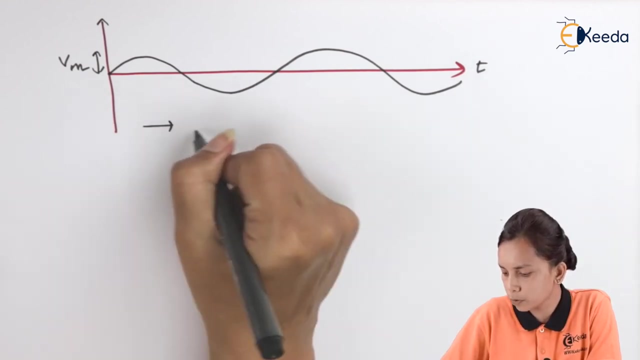 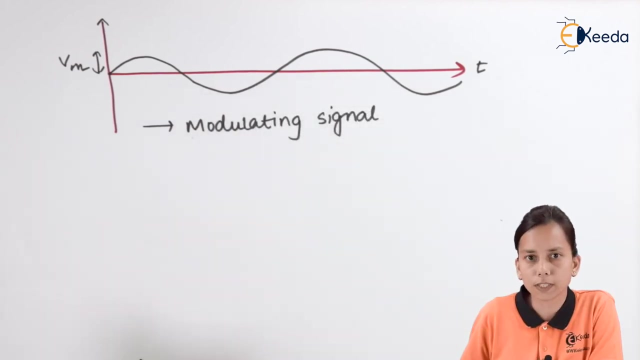 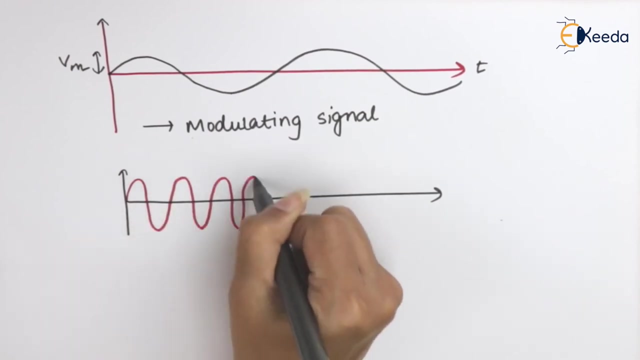 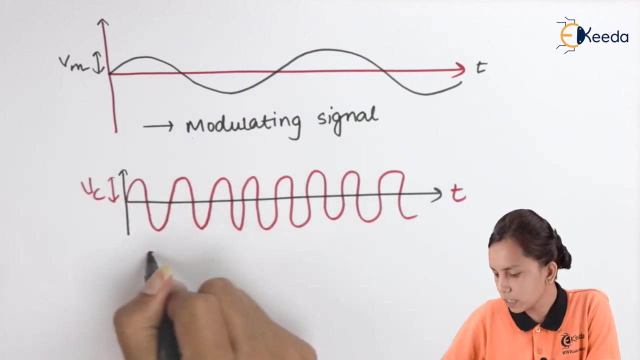 This is our modulating signal, which is of low frequency. that's why I draw it like this, and Let's say it's amplitude is Vm. with respect to time, It is nothing but modulating signal, modulating signal On low-frequency signal. This is our carrier signal. 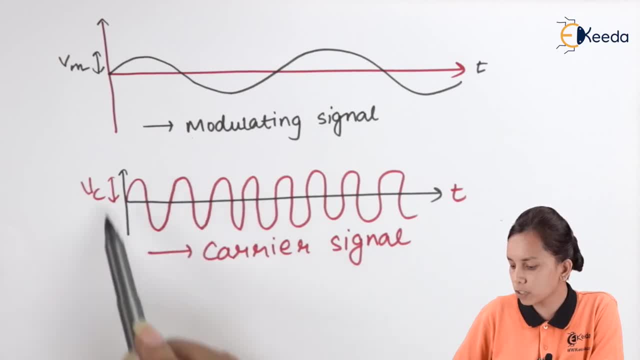 And it is of very high frequency. the frequency of the signal is very high. That's why I draw it like this. now, what we are trying to do, We are trying to represent our modulated signal, amplitude, modulated signal. that how I am saying that my amplitude is. 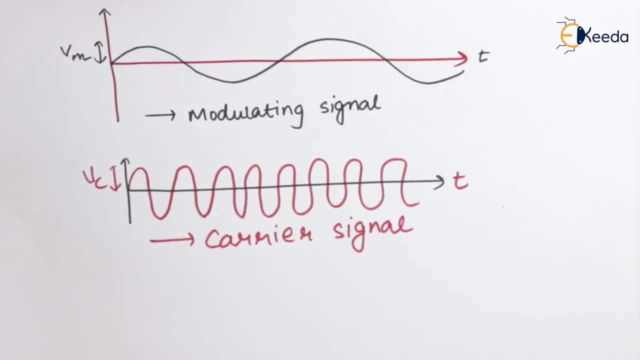 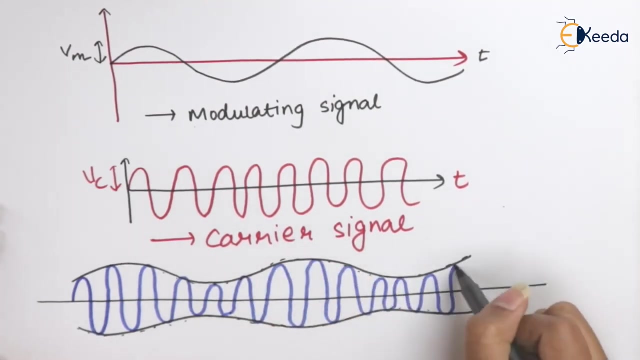 changing with respect to the low frequency signal. and So this is our amplitude modulated signal. this black one, this is a Modulating signal and this blue one is the carrier signal. now look at this whole diagram that every time The amplitude of the carrier signal is changing with respect to the modulating signal. here 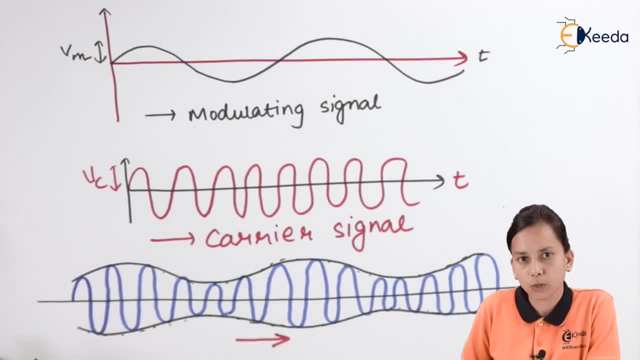 It is low here, It is high, then again low and high. So basically our whole carrier signal is changing with respect to the amplitude of this modulating signal And it is nothing but the representation. Mathematically we can also prove this point. So this is nothing but. the amplitude modulated signal. amplitude modulated signal: There is no change in the frequency of the carrier and there is no change in the phase of the carrier. There's just one change, and that change is actually happening in the amplitude of the carrier. that amplitude is Already changing. at every moment of time the amplitude is changing and this is nothing but the amplitude modulated.